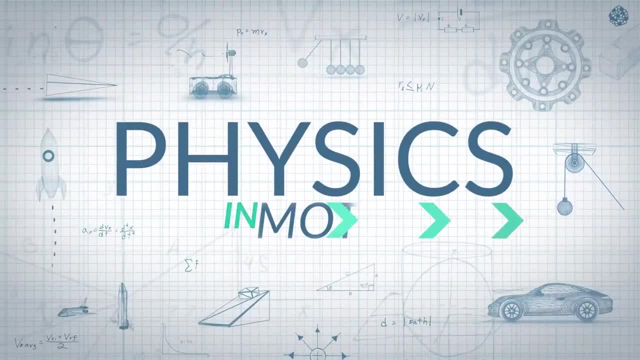 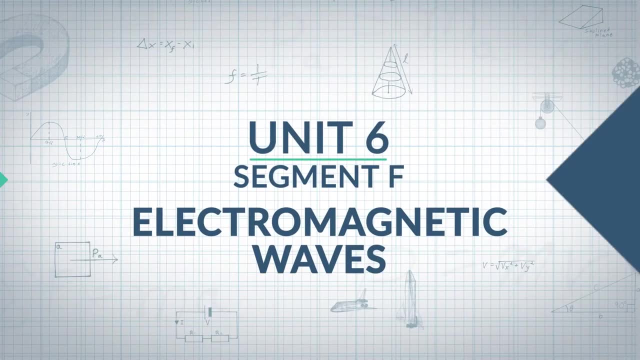 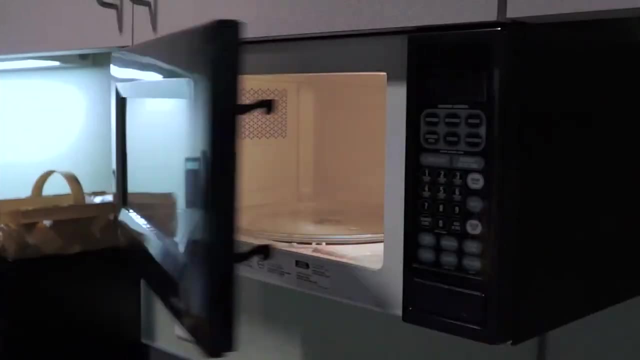 TUNING IN TO YOUR FAVORITE RADIO STATION, LISTENING TO YOUR FAVORITE SONG WHILE EXERCISING, WARMING UP SOME LEFTOVERS IN THE MICROWAVE, OR TALKING ON YOUR CELL PHONE. 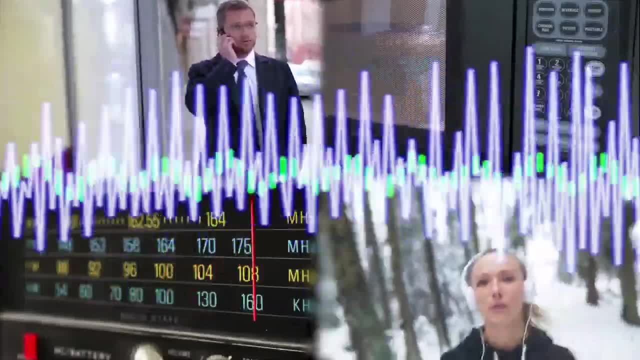 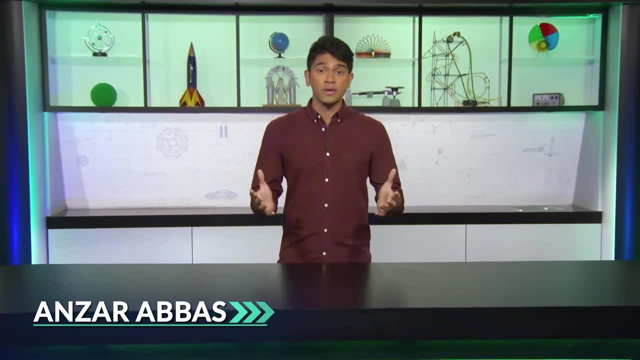 ALL OF THESE ACTIVITIES ARE USING ELECTRO-MAGNETIC WAVES. EM WAVES ARE EVERYWHERE. EM STANDS FOR ELECTRO-MAGNETIC. THE SUN RADIATES ELECTRO-MAGNETIC ENERGY. THIS IS ENERGY THAT TRAVELS THROUGH SPACE. 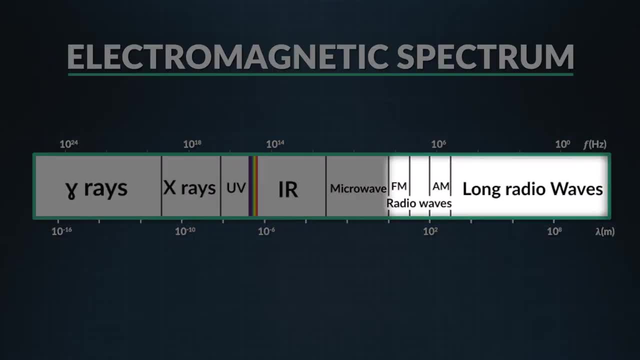 VISIBLE LIGHT IS AN EM WAVE, SO ARE RADIO WAVES, WHOSE WAVELENDS CAN BE MILES LONG. ELECTRO-MAGNETIC WAVES COME IN ALL LENDS AND SIZES AND INCLUDE MICROWAVES, INFRARED RAYS, ULTRA-VIOLET RAYS, X-RAYS AND GAMMA RAYS. 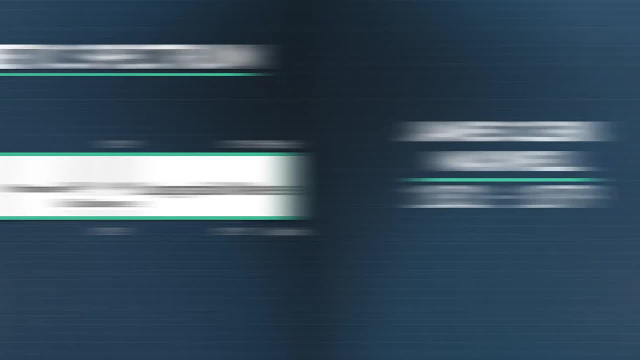 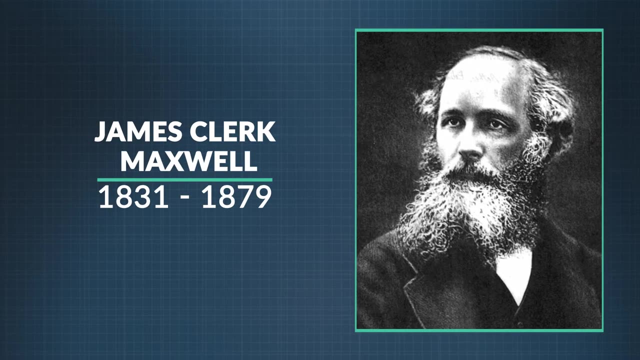 IN WHAT WE CALL THE ELECTRO-MAGNETIC SPECTRUM. IT WAS A SCOTTISH PHYSICIST CALLED JAMES CLARK MAXWELL WHO FIGURED OUT IN AROUND 1865 THAT ELECTRIC AND MAGNETIC FIELDS. 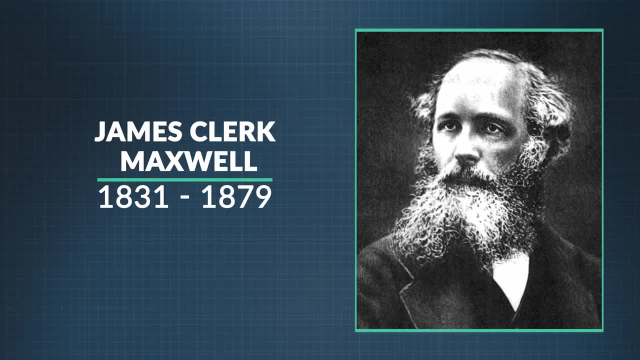 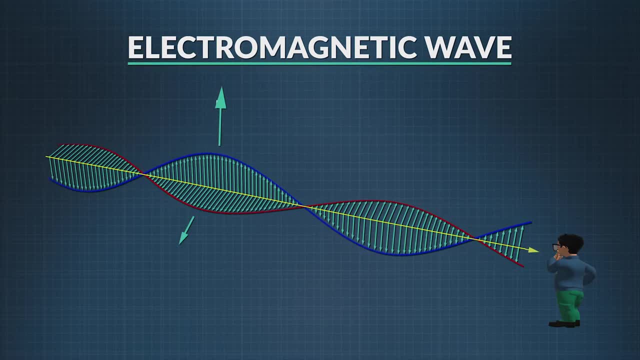 COUPLE TOGETHER TO CREATE WAVES THAT ARE PART OF THE ELECTRO-MAGNETIC SPECTRUM. ELECTRO-MAGNETIC WAVES ARE COMPRISED OF TWO SEPARATE FIELDS: ONE MAGNETIC AND ONE ELECTRIC. 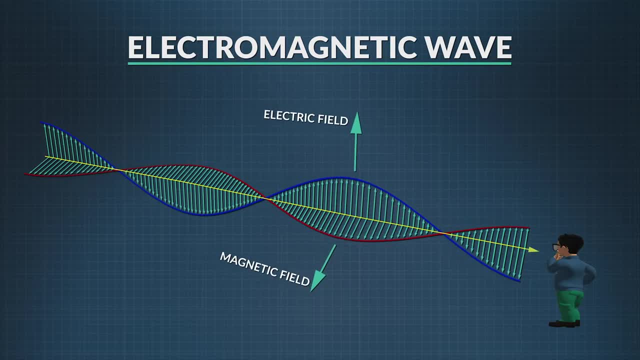 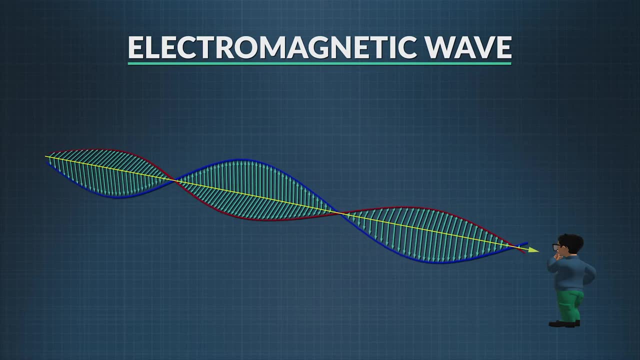 AND THEY'RE PERPENDICULAR TO EACH OTHER. THESE FIELDS INTERACT BECAUSE THEY'RE PART OF THE SAME SYSTEM. THAT MEANS THAT A CHANGING ELECTRIC FIELD CAN CREATE A CHANGING MAGNETIC FIELD AND VICE VERSA. 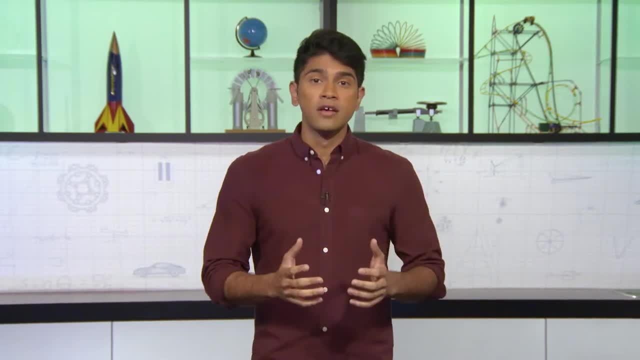 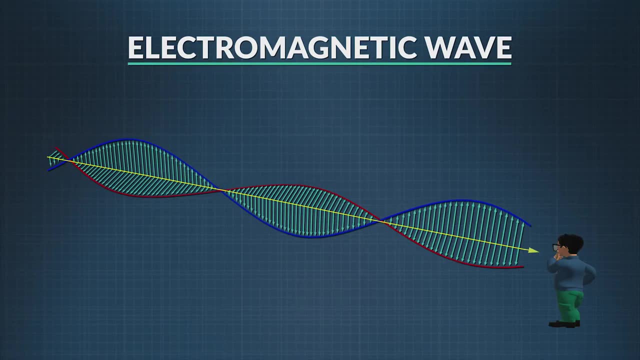 LIGHT WAVES PRODUCE BOTH ELECTRIC AND MAGNETIC FIELDS, SO THEY HAVE BOTH ELECTRIC AND MAGNETIC PROPERTIES IN THIS DIAGRAM. IF THE ELECTRO-MAGNETIC WAVES ARE POINTING, TOWARDS YOU. 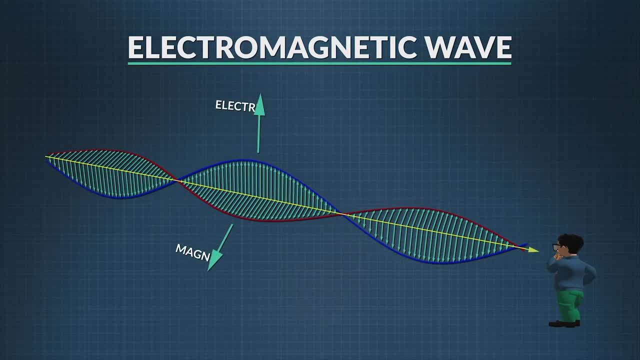 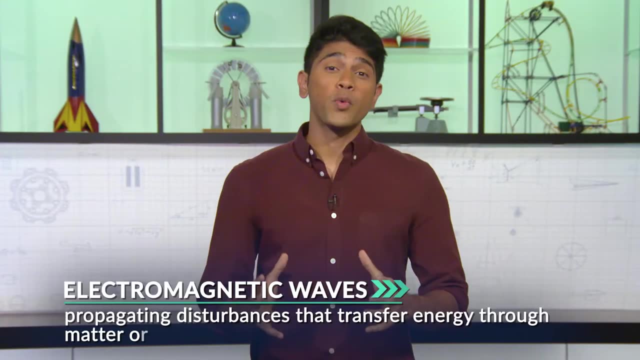 WHICH MEANS THE LIGHT IS SHINING IN YOUR FACE. AND IF THE MAGNETIC FIELD IS OSCILLATING UP AND DOWN, THEN THAT MEANS THE ELECTRIC FIELD IS OSCILLATING LEFT AND RIGHT. ELECTRO-MAGNETIC WAVES ARE PROPAGATING DISTURBANCES. 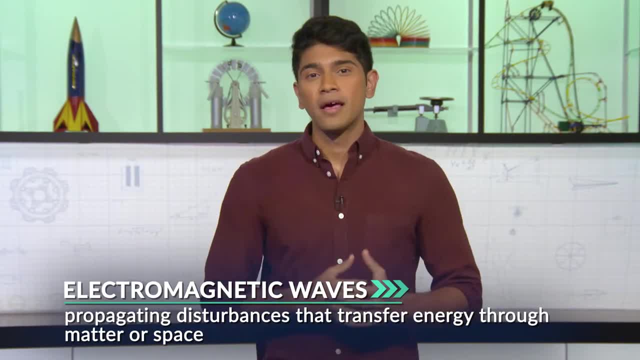 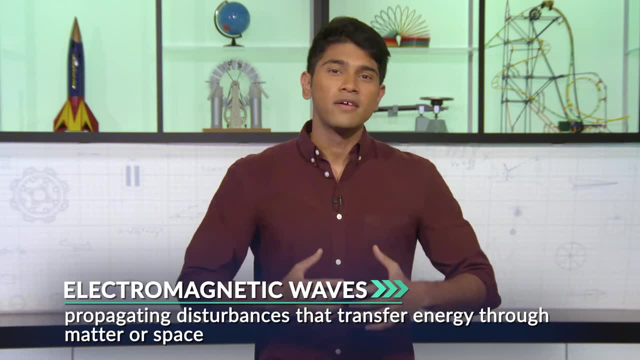 THAT TRANSFER ENERGY THROUGH MATTER OR SPACE. MAXWELL WAS ONE BRILLIANT GUY TO DISCOVER THAT ELECTRIC AND MAGNETIC FIELDS CAN TRAVEL THROUGH SPACE AS WAVES. THIS DISCOVERY CHANGED OUR WORLD. 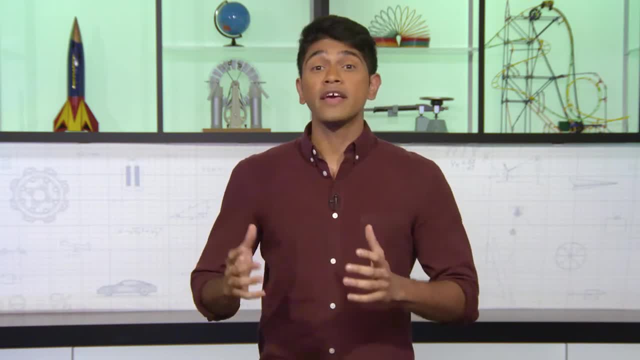 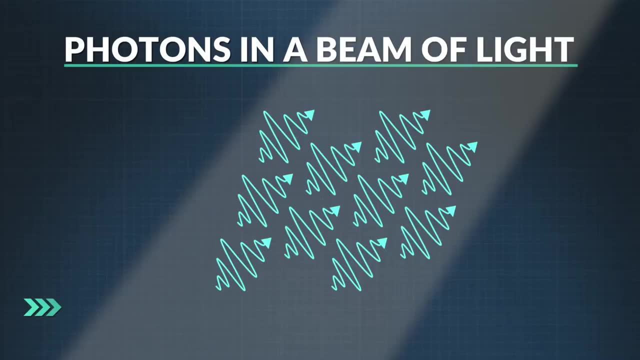 THINK OF ALL WE DO WITH ELECTRO-MAGNETIC WAVES AND UNLIKE OTHER WAVES. ELECTRO-MAGNETIC WAVES EXHIBIT PROPERTIES OF BOTH WAVES AND PARTICLES. THE PARTICLES ARE DISCREET PACKETS OF ENERGY. 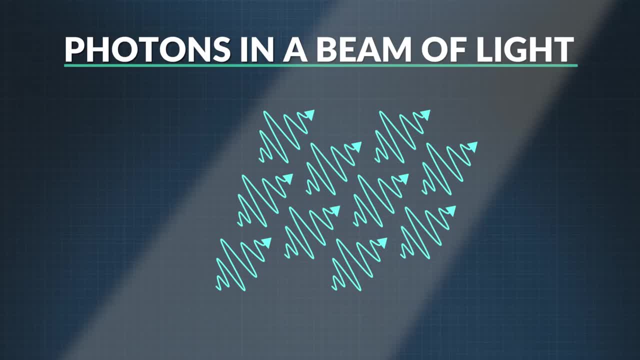 CALLED PHOTONS. YOU CAN ALSO SAY: THESE PHOTONS HAVE VIRTUALLY NO MASS HOWEVER, FROM EINSTEIN'S THEORY OF RELATIVITY, E IS EQUAL TO MC SQUARED. MASS AND ENERGY ARE INTERCHANGEABLE. 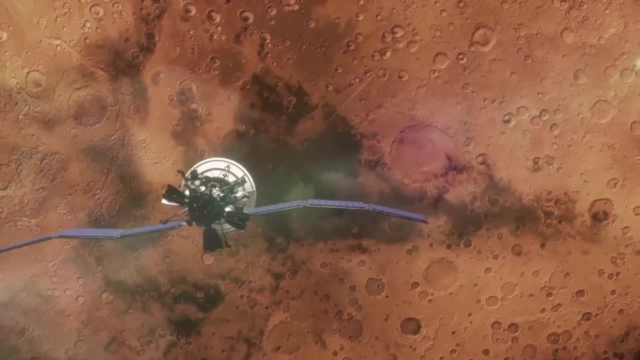 SO IF YOU'RE PLANNING A MISSION TO MARS, FOR EXAMPLE, EVEN THOUGH, IT MAY SEEM INSIGNIFICANT. YOU HAVE TO CALCULATE THE PHOTON PRESSURE FROM RADIATION ON YOUR SPACECRAFT OR YOU'LL MISS YOUR TARGET. 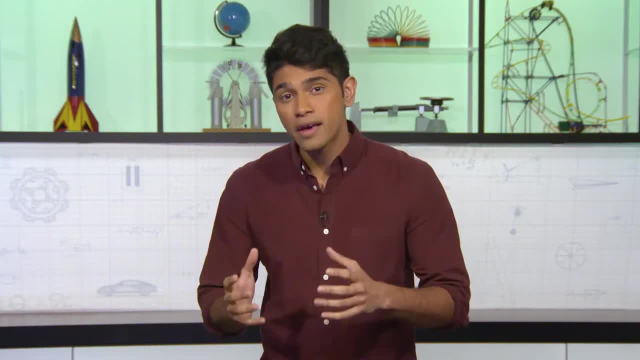 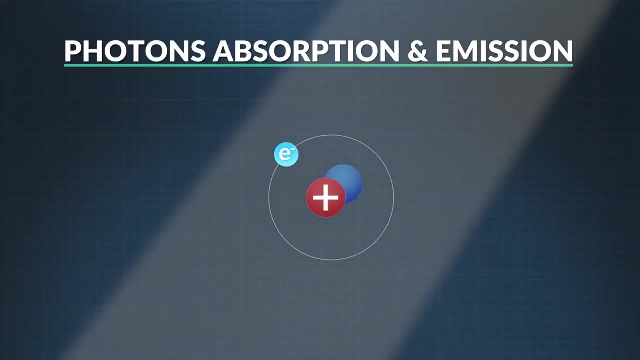 WHEN TRAVELING IN SPACE, THAT MASS CAN MAKE A DIFFERENCE. PHOTONS CAN ALSO EXCITE ELECTRONS. HERE'S AN EXAMPLE: IF YOU SHINE A LIGHT ON GLOW-IN-THE-DARK PAINT, YOU SEE THIS PROCESS IN ACTION. 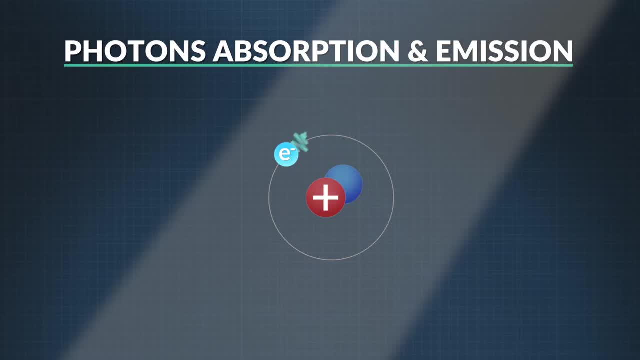 PHOTONS ARE LIGHT AND THE PHOTONS FROM THE FLASHLIGHT EXCITE ELECTRONS IN THE PAINT, CAUSING THE ELECTRONS TO JUMP TO A HIGHER ENERGY LEVEL. AS ELECTRONS FALL BACK TO A LOWER. 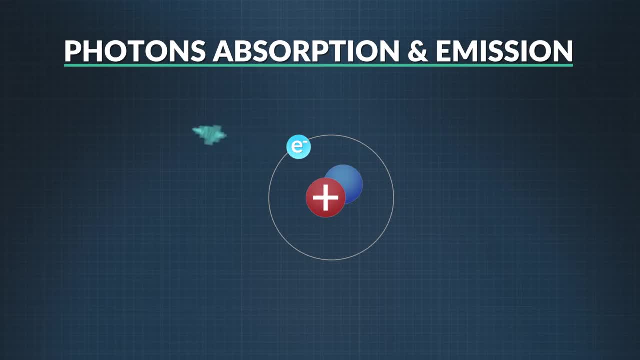 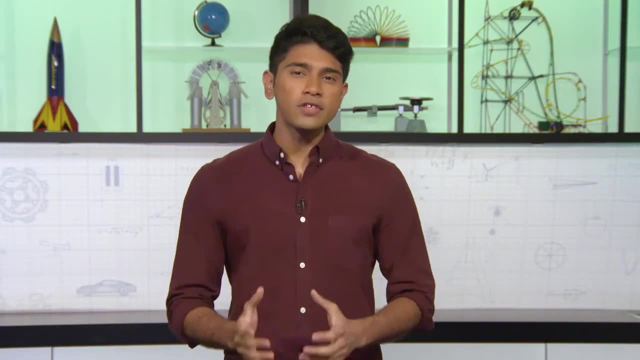 AND MORE STABLE ENERGY LEVEL. THE ELECTRONS EMIT PHOTONS OF LIGHT. THAT'S WHAT CAUSES THE FLORESCENT PAINT TO SHINE. IN 1900, MAX PLANK FIRST INTRODUCED THE IDEA OF LIGHT. 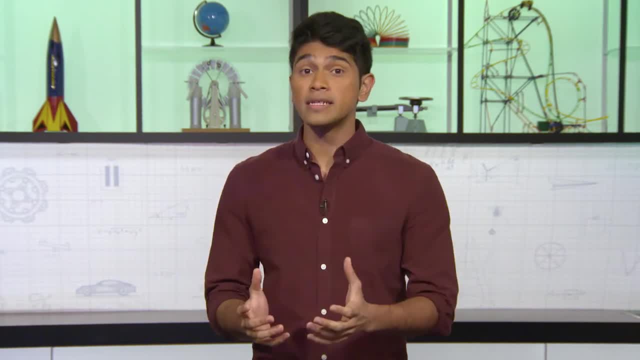 AS PACKETS OF ENERGY, AND IN 1905, ALBERT EINSTEIN PUBLISHED HIS NOBEL PRIZE-WINNING PAPER FURTHERING THE HYPOTHESIS THAT PHOTONS CAN EXCITE ELECTRONS. 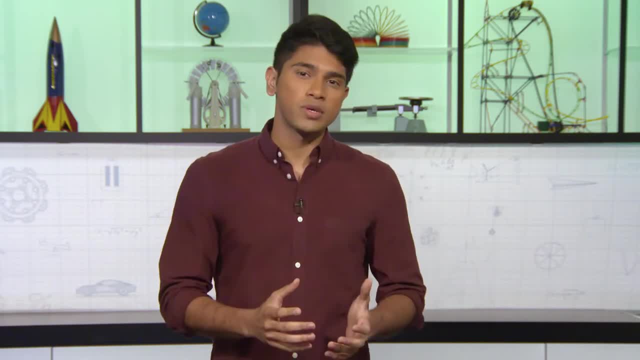 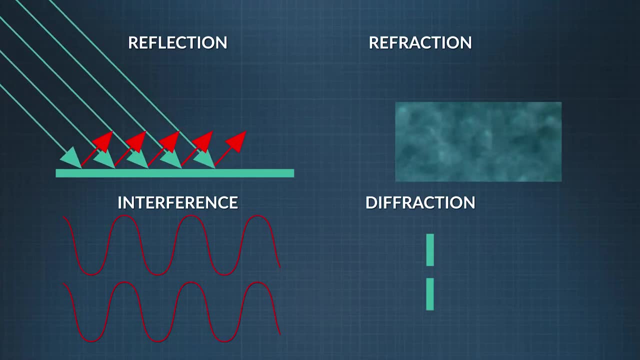 CAUSING THEM TO MOVE BUT UP. UNTIL THE EARLY 20TH CENTURY, IT WAS BELIEVED THAT LIGHT ONLY HAD PROPERTIES OF WAVES AND EXHIBITED THESE PROPERTIES IN FOUR WAYS: REFLECTION, BOUNCING LIGHT OFF OF A SURFACE. 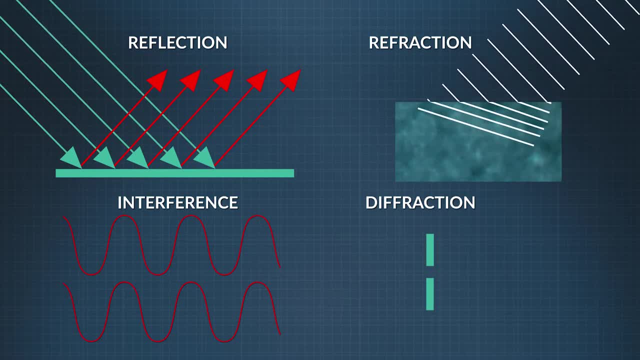 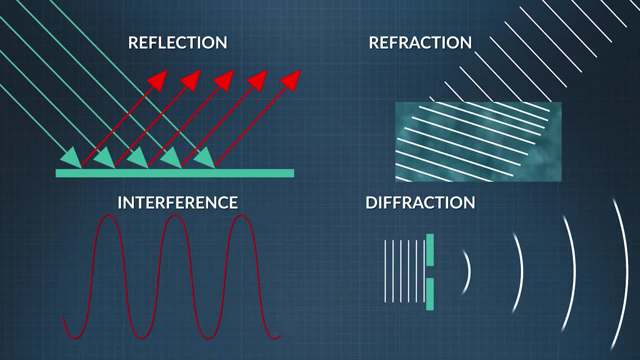 REFRACTION OR THE BENDING OF LIGHT THROUGH A MEDIUM INTERFERENCE, LIGHT WAVES INTERFERING WITH ONE ANOTHER AND DIFFRACTION OR THE BENDING OF LIGHT WAVES AROUND A BARRIER. EINSTEIN'S HYPOTHESIS KNOWN AS 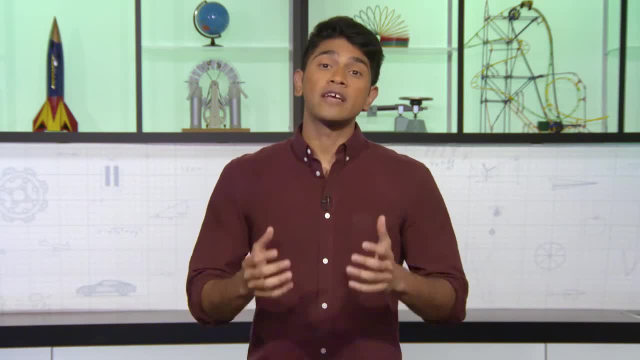 THE PHOTO-ELECTRIC EFFECT BLEW THIS IDEA OUT OF THE WATER IN AN INTERFERENCE DONE BY ROBERT MILLIKEN IN 1914,. THE PHOTO-ELECTRIC EFFECT HYPOTHESIS GAVE US EVIDENCE AS TO THE 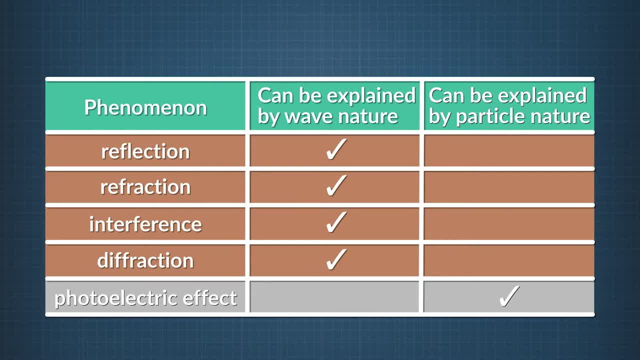 PARTICLE NATURE OF LIGHT, WHILE THE OTHER PHENOMENON SCENE CAN ONLY BE EXPLAINED DUE TO THE WAVE NATURE OF LIGHT. EM WAVES TRANSMIT ENERGY AND THEY CAN TRAVEL IN THE VACUUM OF SPACE. 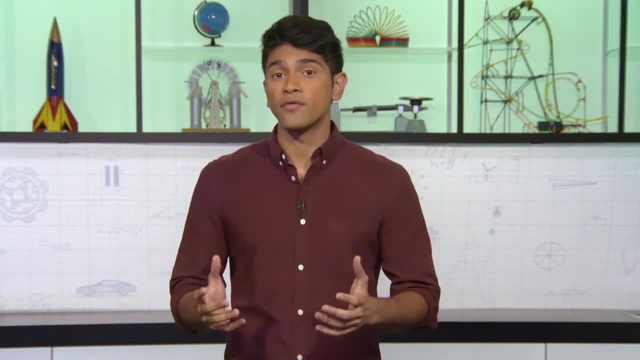 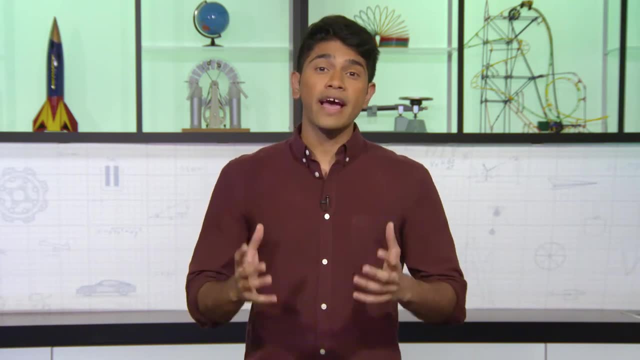 SOUND WAVES TRANSMIT ENERGY, BUT THEY CANNOT TRAVEL IN A VACUUM. THEY NEED A MEDIUM LIKE AIR OR WATER TO TRAVEL. SO DON'T BELIEVE THOSE SCI-FI MOVIES. SPACE IS ACTUALLY A VERY QUIET PLACE. 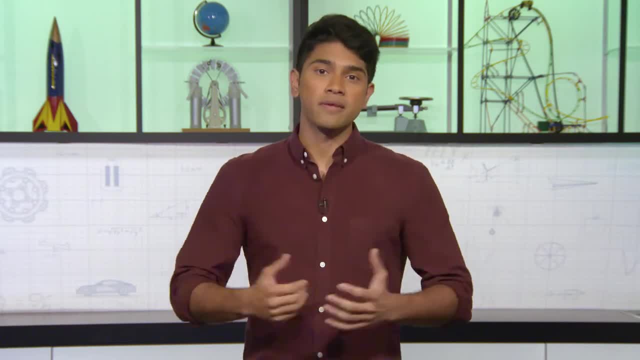 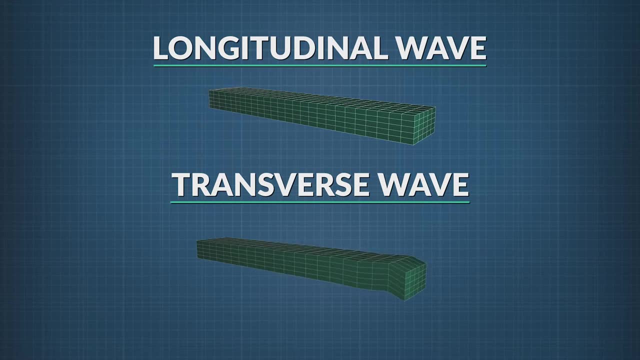 BUT YOU CAN SEE ELECTROMAGNETIC WAVES LIKE STARLIGHT. ANOTHER DIFFERENCE BETWEEN SOUND AND ELECTROMAGNETIC WAVES IS HOW ELECTROMAGNETIC WAVES MOVE. A SOUND WAVE IS LONGITUDINAL, THE MEDIUM THROUGH WHICH THE WAVE TRAVELS. 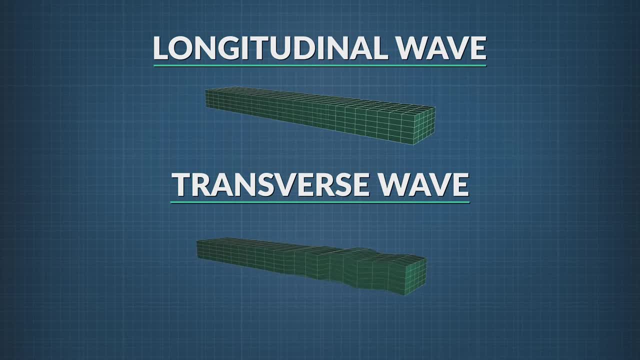 IS IN THE SAME DIRECTION OF THE FORCE THAT FIRST PROPELLED IT. AN ELECTROMAGNETIC WAVE IS A TRANSVERSE WAVE. THAT MEANS THE MEDIUM THROUGH WHICH THE WAVE TRAVELS MOVES PERPENDICULAR TO THE DIRECTION. 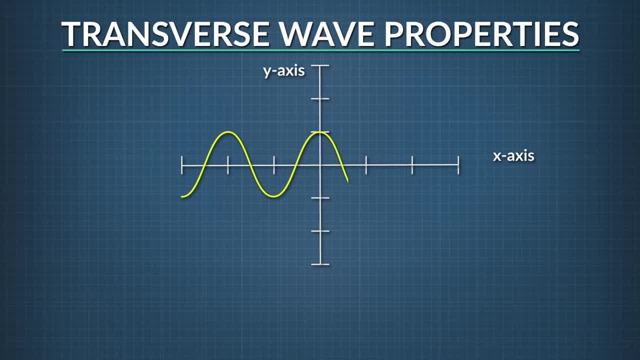 THE WAVE IS TRAVELING. ALL TRANSVERSE WAVES, LIKE ELECTROMAGNETIC WAVES, HAVE THESE PROPERTIES. THE TROUGH IS THE LOWEST POINT OF A TRANSVERSE WAVE. THE CREST IS THE HIGHEST POINT OF A TRANSVERSE WAVE. 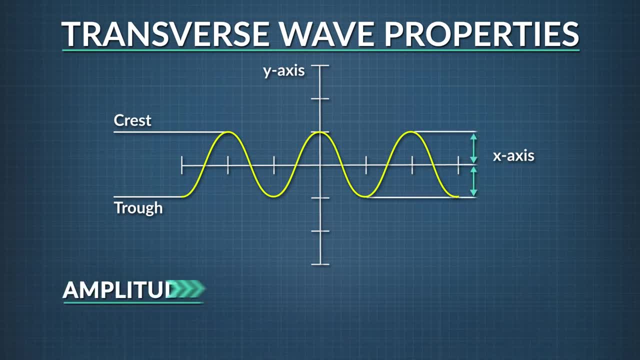 IF YOU DRAW A VERTICAL LINE FROM THE VERY TIP OF THE CREST TO THE EQUILIBRIUM POINT, OR THE BOTTOM OF A TROUGH TO THE EQUILIBRIUM POINT, THAT'S CALLED AMPLITUDE, AND A WAVELENTH IS MEASURED AS: 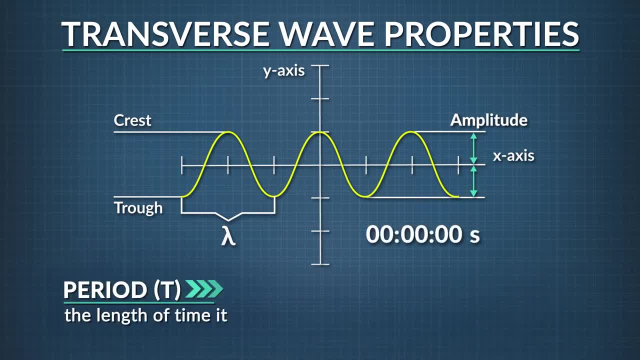 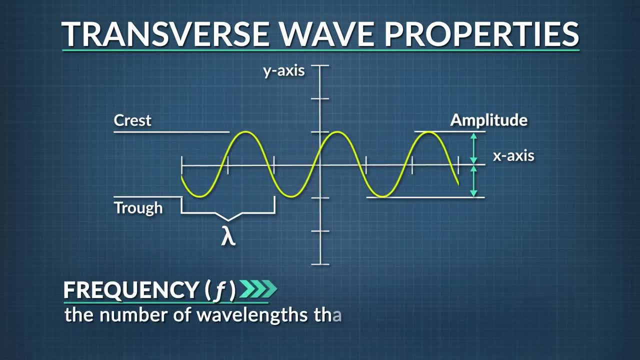 ONE COMPLETE CREST AND ONE COMPLETE TROUGH. THE PERIOD T IS THE LENGTH OF TIME IT TAKES FOR A WAVELENTH TO PASS BY A GIVEN POINT IN SPACE MEASURED IN SECONDS, THE FREQUENCY OF ELECTROMAGNETIC WAVES. 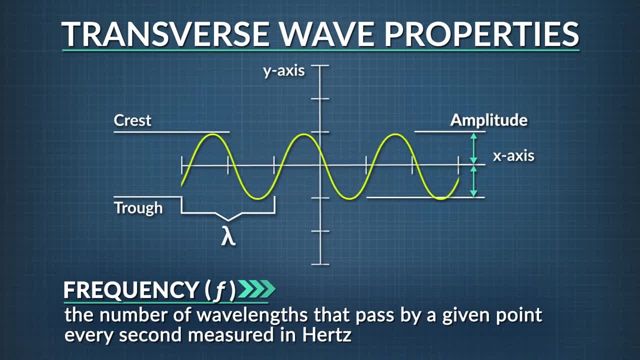 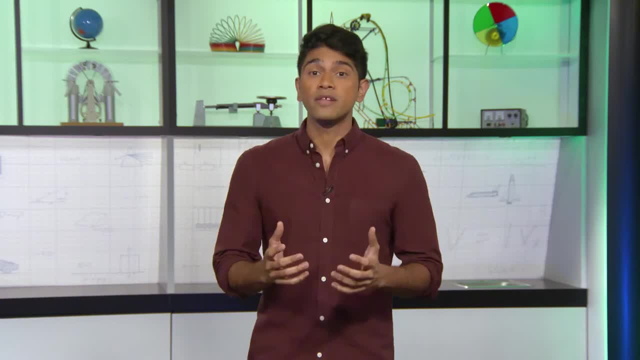 LIKE ALL WAVES IS THE NUMBER OF WAVELENDS THAT PASSES A POINT IN A SECOND MEASURED IN HURTS, SINCE THE FREQUENCY IS THE NUMBER OF WAVES PASSING A GIVEN POINT IN A SECOND, THAT IS WAVELENDS PER TIME. 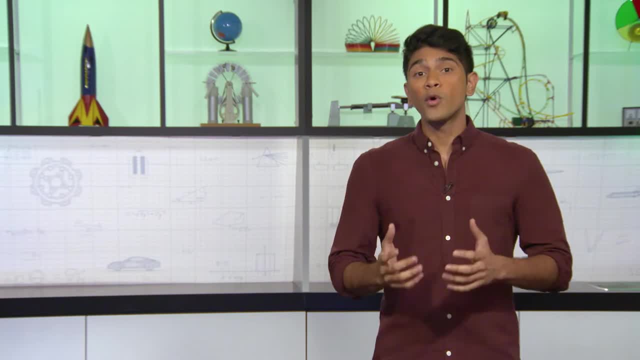 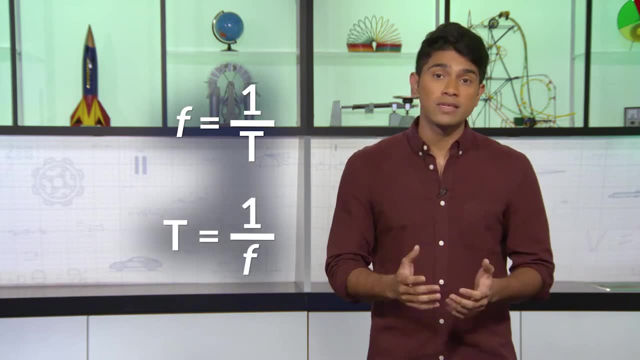 THE FREQUENCY IS EQUAL TO ONE WAVE PER ITS PERIOD, OR FREQUENCY EQUALS ONE DIVIDED BY THE PERIOD T. SIMILARLY, PERIOD IS EQUAL TO ONE OVER ITS FREQUENCY F. IN THIS GRAPHIC YOU CAN SEE THE RELATIONSHIP. 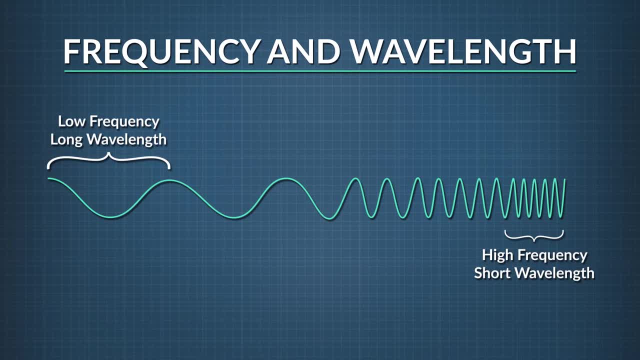 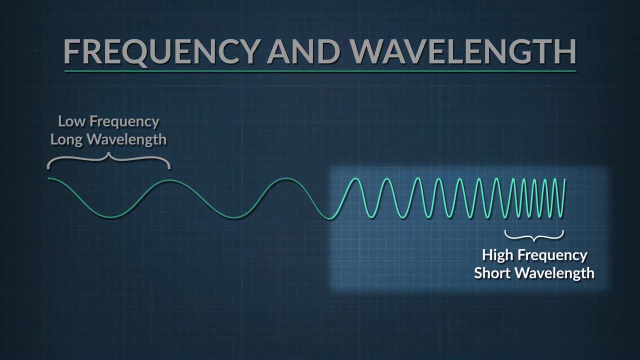 BETWEEN WAVELENTH AND FREQUENCY. SINCE LIGHT TRAVELS AT A CONSTANT SPEED. IF THE FREQUENCY OF THE WAVE INCREASES, THE LENGTH OF THE WAVE DECREASES, SO SHORTER. WAVELENDS HAVE HIGHER FREQUENCIES. 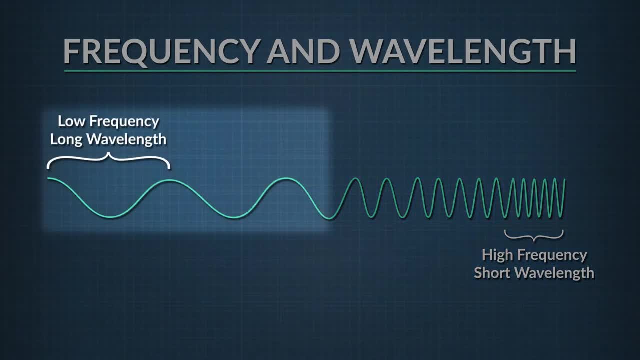 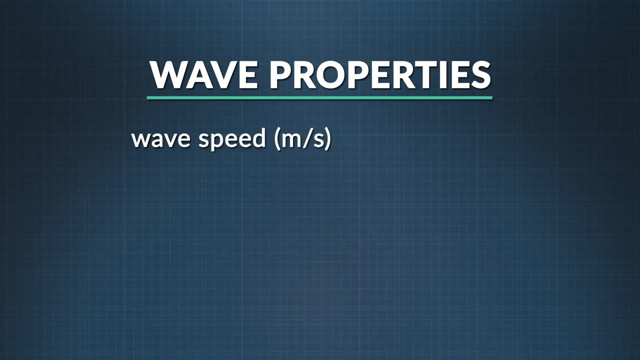 AND LONGER. WAVELENDS, LIKE RADIO WAVES, HAVE LOWER FREQUENCIES, SO WAVELENDS AND FREQUENCY ARE INVERSELY PROPORTIONAL. WE TYPICALLY MEASURE THE SPEED OF WAVE IN METERS PER SECOND AND WRITE IT. 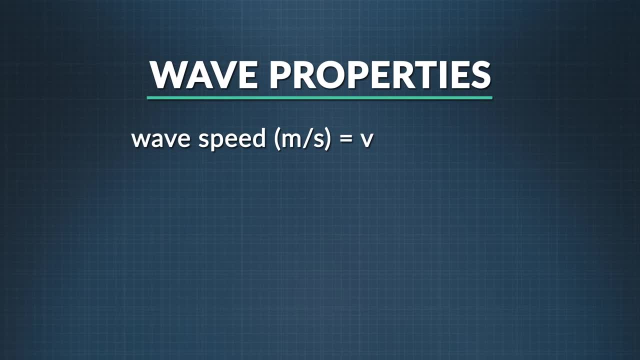 AS A SMALL V. THE VELOCITY OF LIGHT IS A SPECIAL CASE. WE WRITE THE SPEED OF LIGHT IN VACUUM AS A LOWER CASE. C IT'S THE SPEED OF LIGHT MEASURED IN METERS PER SECOND, AND REMEMBER FREQUENCY IS A SMALL F. 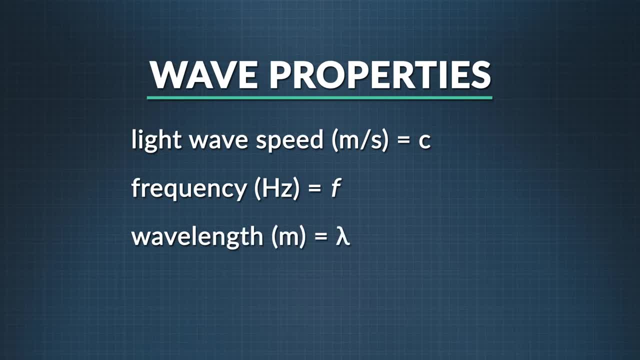 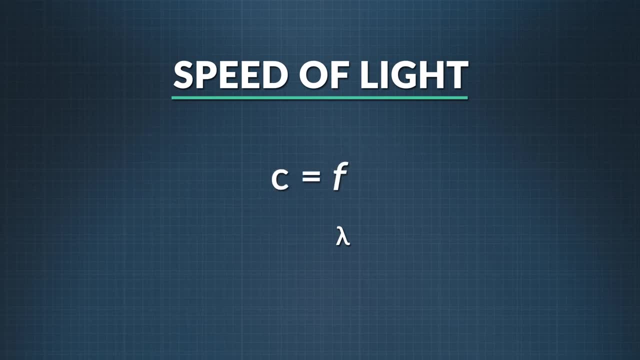 MEASURED IN HURTS, AND WAVELENTH IS LAMBDA MEASURED IN METERS. SO THE SPEED OF LIGHT IN METERS PER SECOND IS EQUAL TO THE FREQUENCY OF THE WAVE MEASURED IN HURTS TIMES, ITS WAVELENTH MEASURED IN METERS. 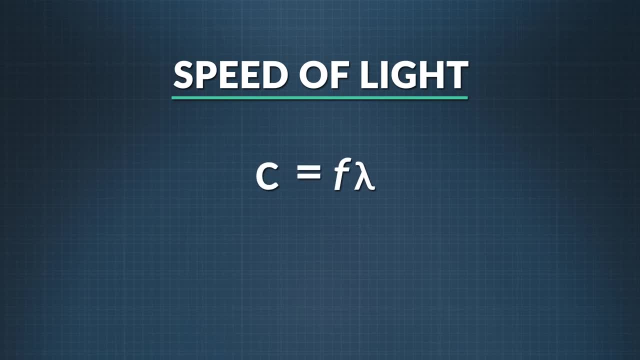 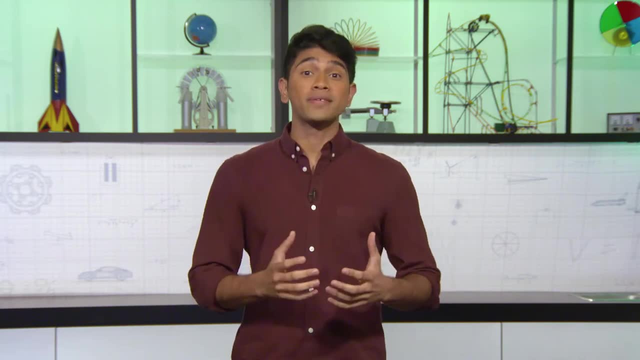 SIMPLY WRITTEN, C EQUALS F TIMES LAMBDA. WHEN AN ELECTRO-MAGNETIC WAVE IS TRAVELING IN THE VACUUM OF SPACE, ITS SPEED C IS ALWAYS THE SAME, AND GUESS WHAT THAT IS. 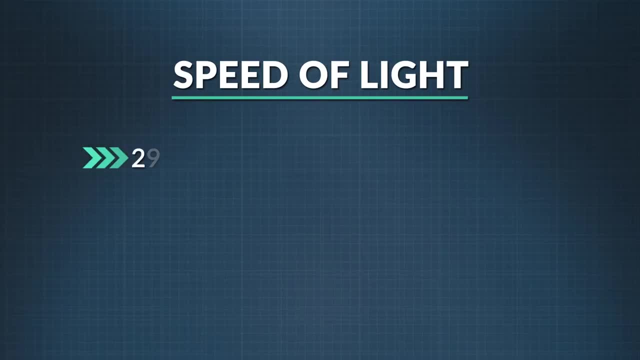 IT'S THE SPEED OF LIGHT, WHICH IS 299,792,458 METERS PER SECOND, OR 670,616,629 MILES PER HOUR. THAT'S WHAT YOU WILL USE IN AN EQUATION TO FIND THE FREQUENCY OF AN ELECTRO-MAGNETIC WAVE. 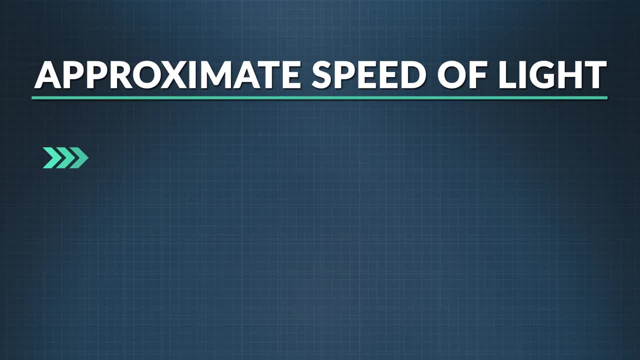 OKAY, TO MAKE IT A LITTLE EASIER. WE USUALLY ROUND IT TO 300 MILLION OR THREE TIMES. TEN TO THE EIGHTH, METERS PER SECOND. KEEP IN MIND THAT THIS NUMBER IS FOR LIGHT IN A VACUUM. 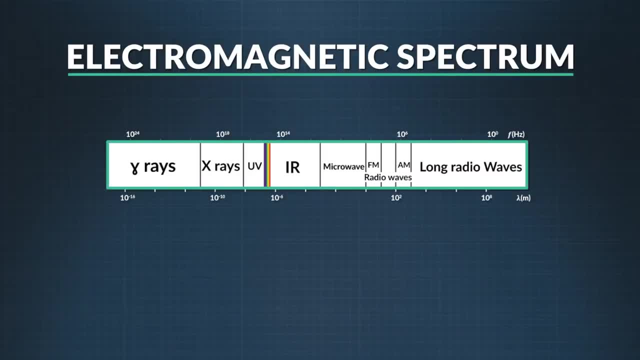 IT CAN BE SLOWER IF LIGHT MOVES THROUGH DIFFERENT MEDIUMS. OKAY, LET'S GO BACK TO THE ELECTRO-MAGNETIC SPECTRUM, SHOWING THE VARIETY OF ELECTRO-MAGNETIC WAVES. 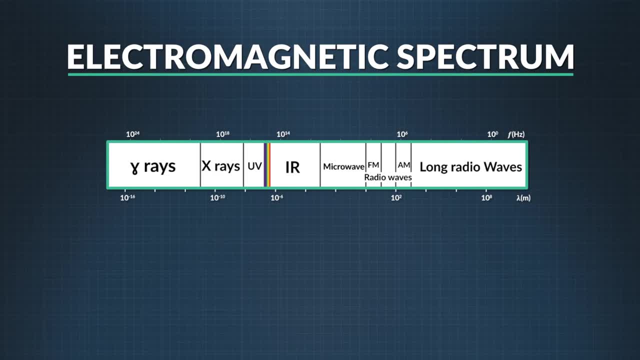 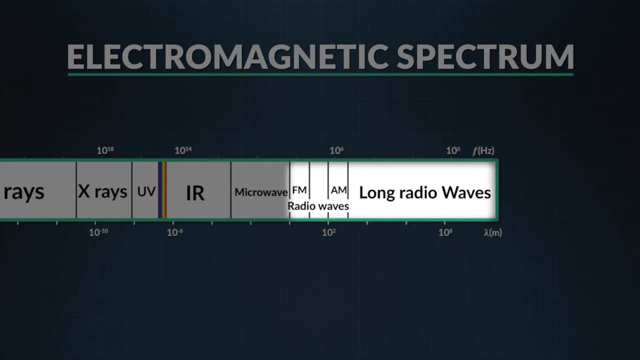 WHAT SETS EACH TYPE OF WAVE APART ON THE SPECTRUM IS ITS WAVELENTH. ON THE RIGHT END ARE THE RADIO WAVES, THE LONGEST WAVES WITH THE LOWEST FREQUENCIES OF THE SPECTRUM. 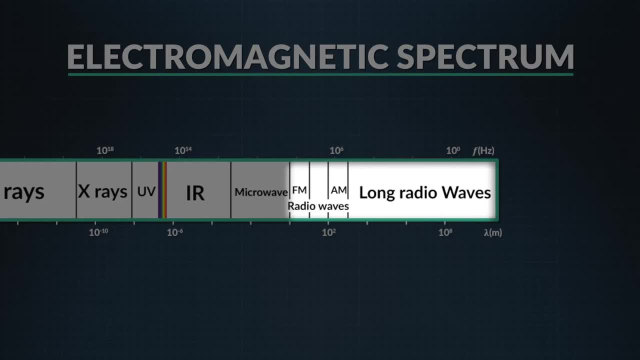 THEIR WAVELENDS CAN BE FROM ONE CENTIMETER TO MORE THAN A KILOMETER IN LENGTH. THESE WAVES ARE TRANSMITTED INTO DIFFERENT BANDS THAT HAVE DIFFERENT PRACTICAL USES- VHF AND UHF WAVES, FOR EXAMPLE. 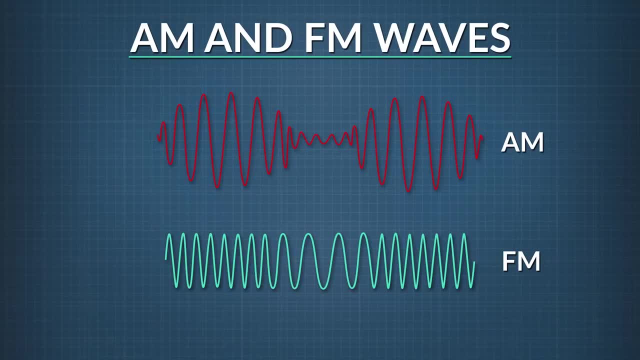 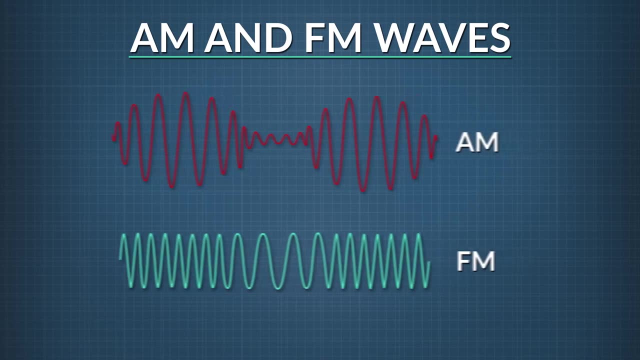 ARE USED TO TRANSMIT TELEVISION SIGNALS. THE LOWER FREQUENCY RADIO WAVES THAT CAN BE THE LENGTH OF A FOOTBALL FIELD ARE WHAT AM AND FM RADIO STATIONS USE TO BROADCAST, BY THE WAY, AM STANDS FOR AMPLITUDE MODULATION. 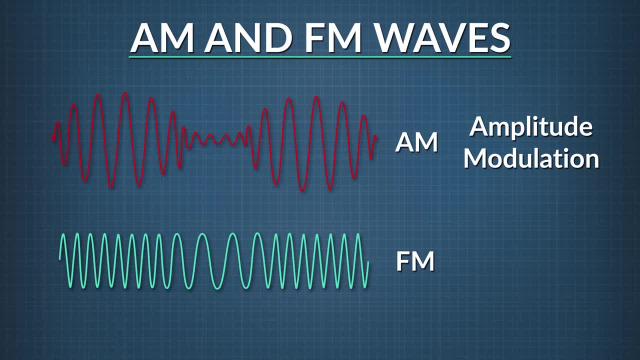 THOSE RADIO STATIONS, VARY THE AMPLITUDE OF THE SIGNALS ACROSS A CARRIER WAVE AND FM STATIONS, VARY THE FREQUENCIES ACROSS THE CARRIER SIGNAL. THAT'S WHY FM STANDS FOR FREQUENCY MODULATION. 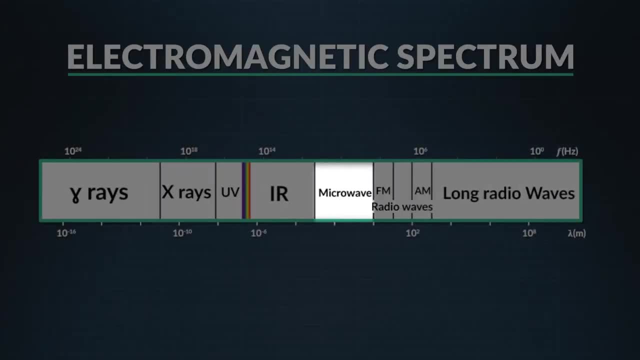 AS YOU MOVE LEFT ON THIS SPECTRUM, THEN THERE ARE MICROWAVES. WAVELENDS IN THIS PART OF THE SPECTRUM CAN RANGE FROM THE RADIO RANGE AROUND ONE METER IN LENGTH, ALL THE WAY TO THE INFRARED RANGE. 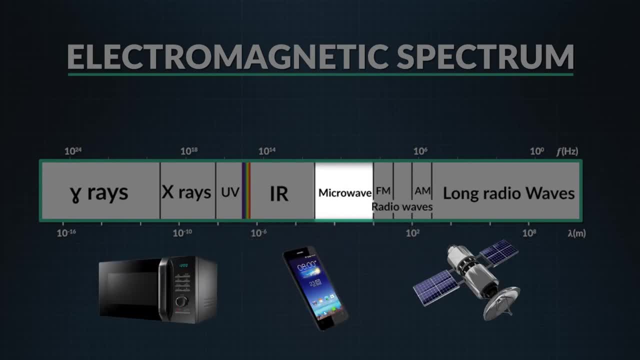 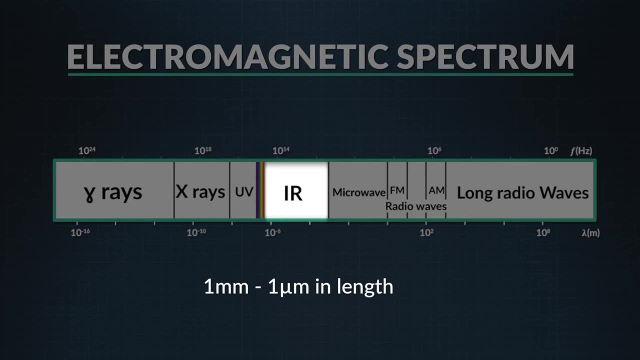 LESS THAN ONE MILLIMETER IN LENGTH. MICROWAVE OVENS, CELL PHONES AND COMMUNICATION SATELLITES ALL USE MICROWAVES. NEXT ARE INFRARED WAVES WITH WAVELENDS FROM ONE MILLIMETER. 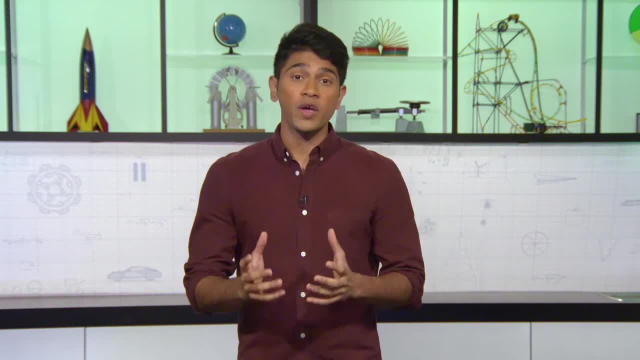 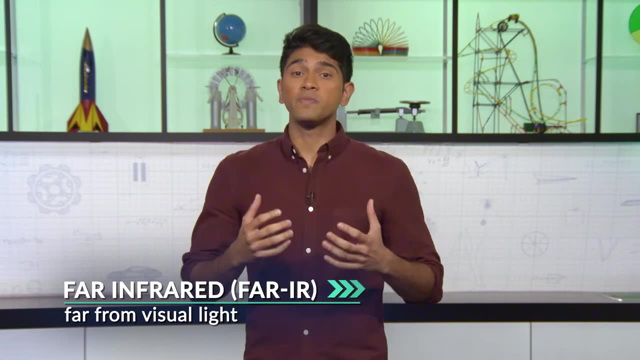 ALL THE WAY DOWN TO THE TINY LENGTH OF ONE MILLIMETER IN LENGTH, INFRARED WAVES THAT LIE CLOSER TO THE MICROWAVE PART OF THE SPECTRUM, ARE CALLED FAR-INFRARED MEANING IT'S FAR FROM VISUAL LIGHT. 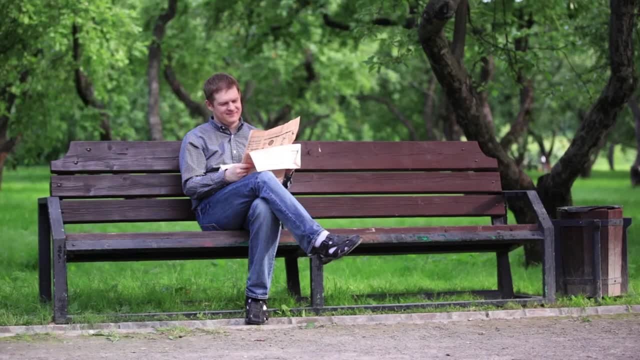 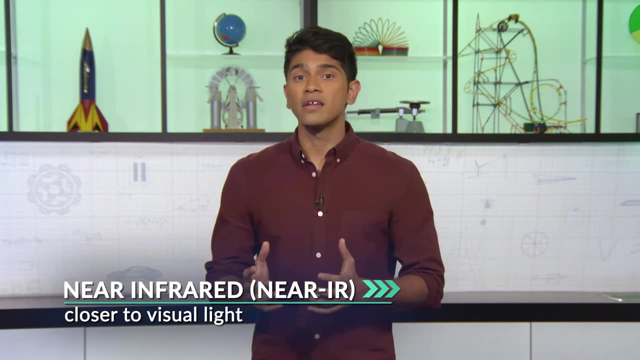 THIS IS THE TYPE OF RADIATION WE EXPERIENCE AS HEAT, THE HEAT WE FEEL FROM A FIRE, FROM SUNLIGHT OR A WARM PARK BENCH IS IN THIS RANGE OF THE INFRARED SPECTRUM, SHORTER NEAR-INFRARED WAVES. 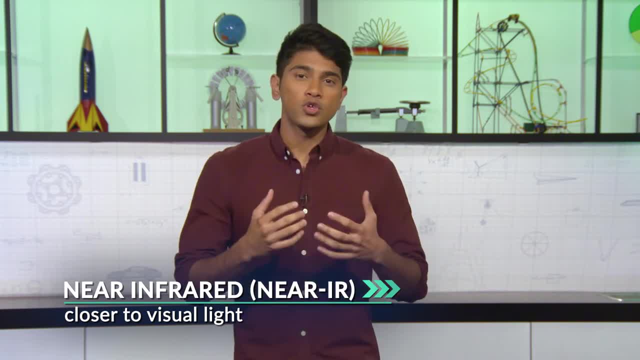 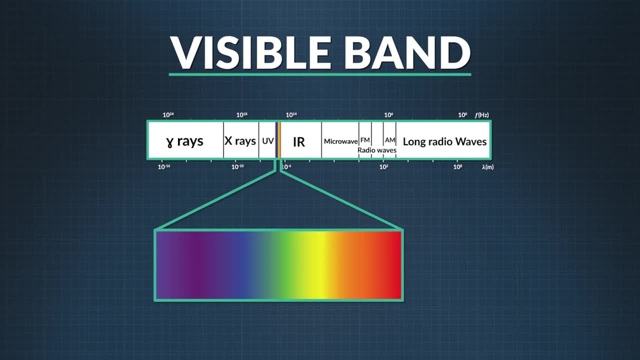 WHICH ARE CLOSER TO VISUAL LIGHT ARE NOT HOT AT ALL. IN FACT, YOU CAN'T EVEN FEEL THEM OR SEE THEM. LOOKING AROUND THE MIDDLE SECTION OF THE SPECTRUM, WE CAN ACTUALLY SEE THESE WAVES. 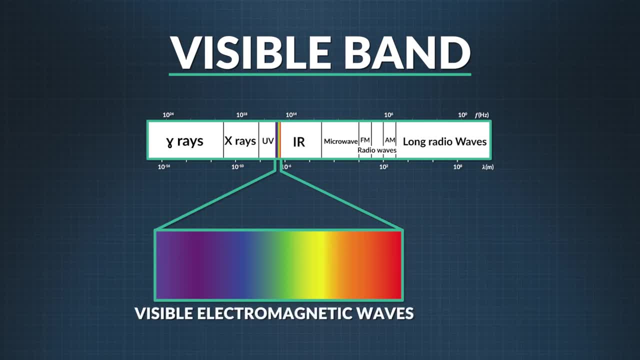 WITH OUR NAKED EYE. THEY'RE THE VISIBLE ELECTRO-MAGNETIC WAVES. RED IS A LONGER WAVE LENGTH AROUND 700 NANOMETERS AND A LOWER FREQUENCY WAVE COMPARED TO VIOLET. 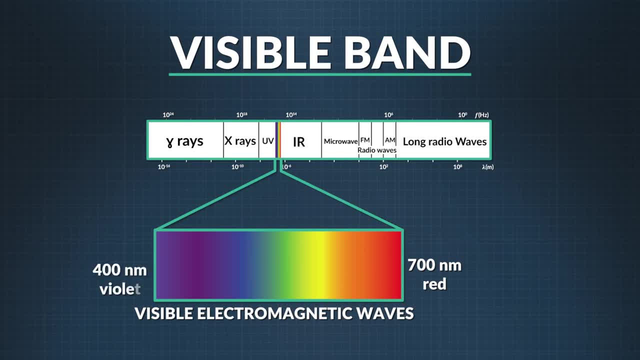 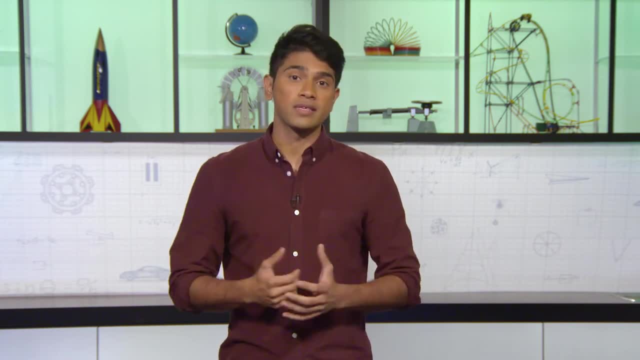 THAT IS A SHORTER WAVE. LENGTH VIOLET IS A HIGHER FREQUENCY WAVE OF ABOUT 400 NANOMETERS AFTER THE VISIBLE PART OF THE ELECTRO-MAGNETIC SPECTRUM ARE ULTRA-VIOLET WAVES. 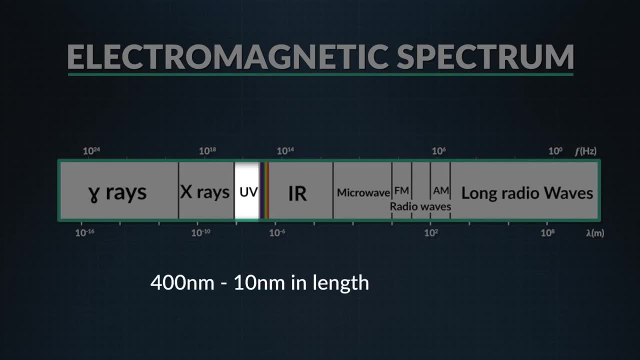 ON THE HIGHER FREQUENCY SIDE, THEY ARE BETWEEN 400 NANOMETERS AND 10 NANOMETERS. THESE ARE MORE DANGEROUS WAVES, WHY BECAUSE? THE HIGHER THE FREQUENCY, THE MORE ENERGIZED THE WAVES. 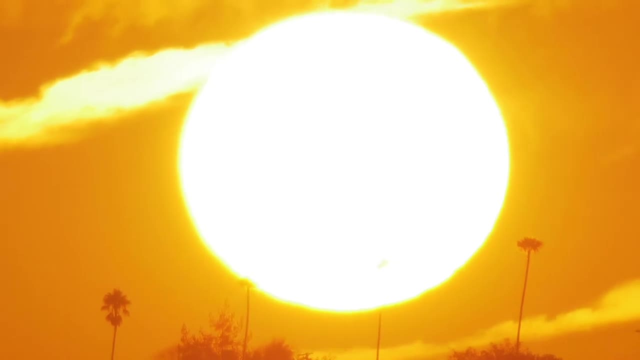 AND THE MORE THEY CAN PENETRATE LIVING CELLS. THESE WAVES ARE WHAT CAN CAUSE SUN TANS AND, IF RECEIVED IN LARGE AMOUNTS, CAN CAUSE SUN BURN OR EVEN SKIN CANCER. THAT'S WHY WE WEAR SUNSCREEN. 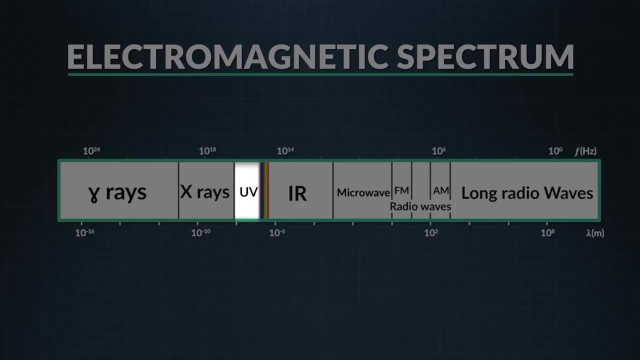 TO SHIELD OUR BODIES FROM ULTRA-VIOLET RAYS, AND THERE ARE EVEN HIGHER FREQUENCY RAYS, X-RAYS- WHICH HAVE A WAVELENSE BETWEEN 100 NANOMETERS AND 0.01 NANOMETERS. 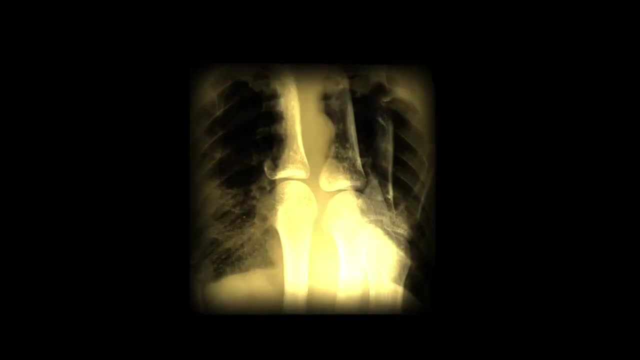 THESE CAN PENETRATE THROUGH OUR SKIN AND MUSCLE LAYERS, BUT NOT OUR BONES. THAT'S HOW WE CAPTURE IMAGES OF OUR BONES, BECAUSE X-RAYS CAN ALSO PENETRATE OUR ORGANS. 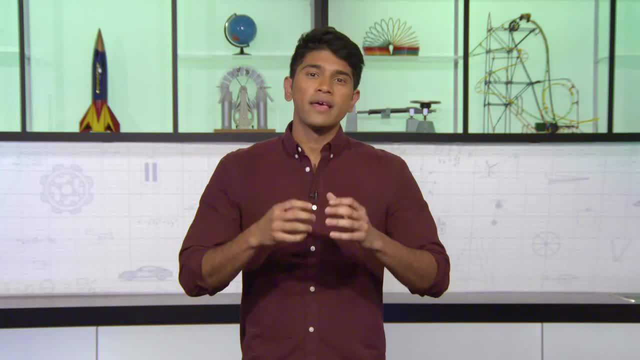 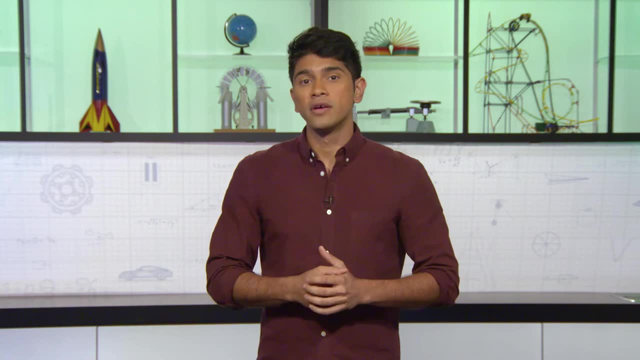 WE LIMIT THE AMOUNT OF X-RAYS, WE RECEIVE GAMMA. RAYS HAVE AN EVEN HIGHER FREQUENCY AND SHORTER WAVELENSE THAN X-RAYS WITH WAVELENSE LESS THAN ONE PICOMETER, SO THEY'RE EVEN MORE ENERGETIC. 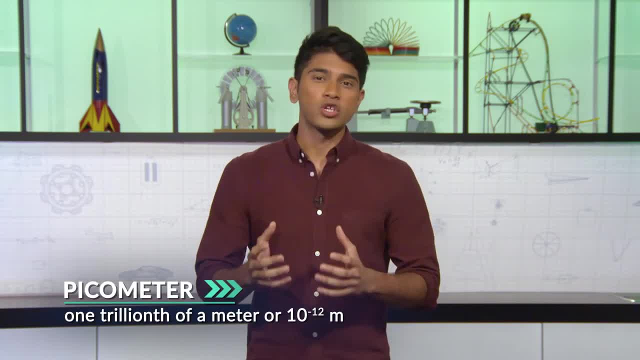 AND DANGEROUS. A PICOMETER, BY THE WAY, IS ONE TRILLIONTH OF A METER OR ONE TWELVETH METERS. ATOMS ARE BETWEEN 60 AND 520 PICOMETERS IN DIAMETER. 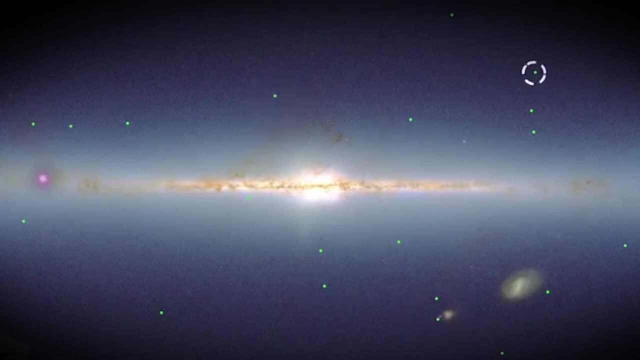 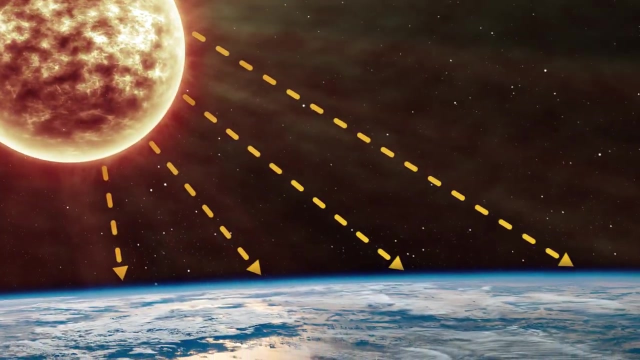 GAMMA RAYS ARE CREATED IN NUCLEAR REACTIONS, IN SPACE OR IN THE LAB. THE EARTH IS CONSTANTLY EXPOSED TO SMALL AMOUNTS OF GAMMA RAYS. FOR EXAMPLE, THEY'RE FOUND IN SOLAR FLAYERS. 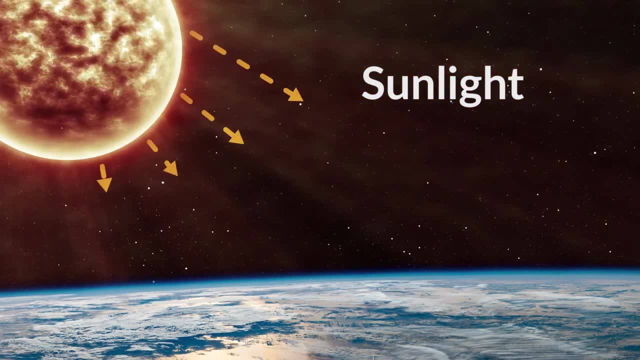 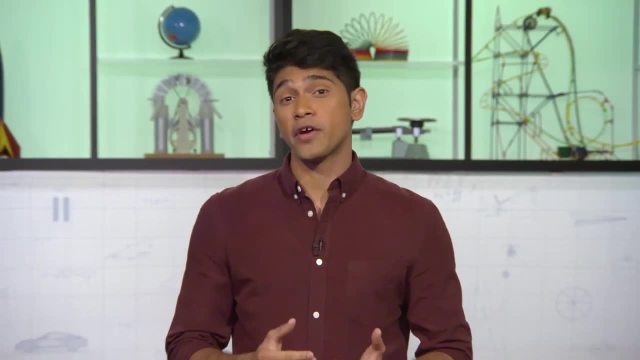 AND SUPERNOVAE THANKFULLY. THE EARTH'S ATMOSPHERE ABSORBS MOST OF THE X-RAYS AND GAMMA RAYS FROM SPACE LAB. TECHNICIANS WHO WORK WITH THESE HIGH-ENERGY WAVES MUST STAND BEHIND PROTECTIVE BARRIERS. 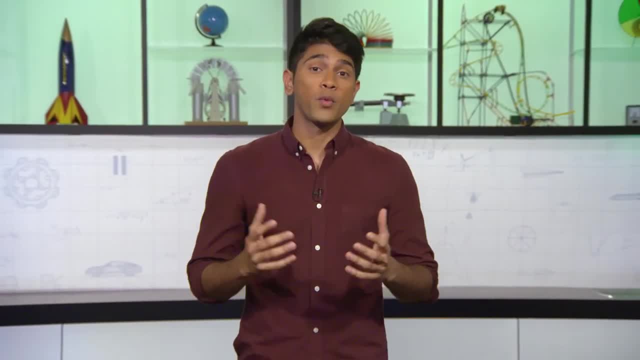 SO NOW YOU'VE SEEN THE ELECTROMAGNETIC SPECTRUM AND ALL OF ITS ELECTROMAGNETIC WAVES- EM WAVES- ALLOW US TO DO SOME AMAZING THINGS, LIKE SEE COLORS, SEND COMMUNICATION SIGNALS. 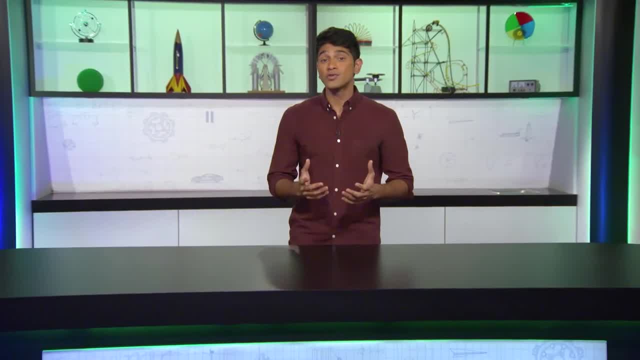 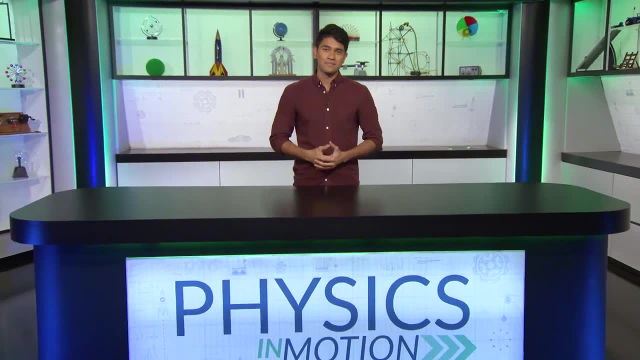 AROUND THE WORLD TALK ON CELL PHONES THAT EVEN PENETRATE TISSUE TO SEE BONES. THAT'S IT FOR THIS SEGMENT OF PHYSICS IN MOTION AND WE'LL SEE YOU NEXT TIME FOR MORE PRACTICE PROBLEMS. 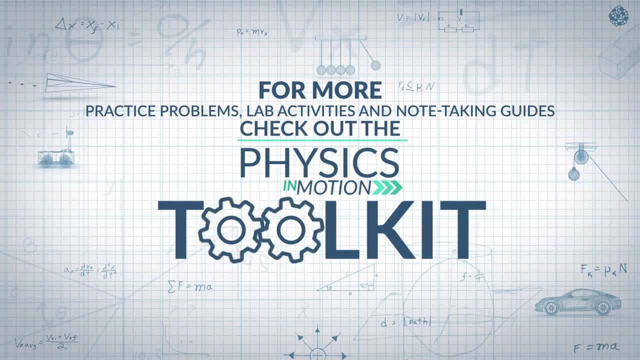 LAB ACTIVITIES AND NOTE-TAKING GUIDES. CHECK OUT THE PHYSICS IN MOTION TALK-IT. 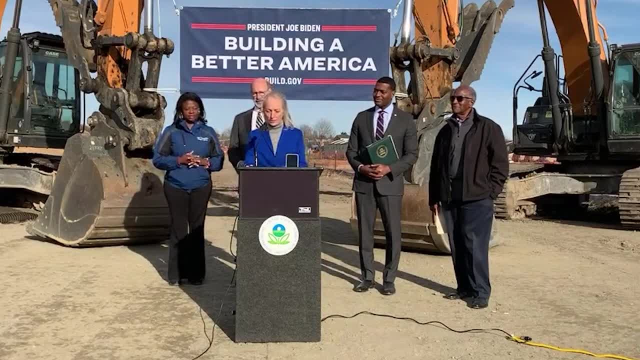 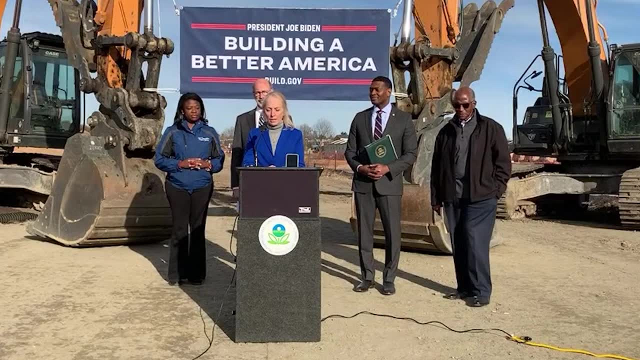 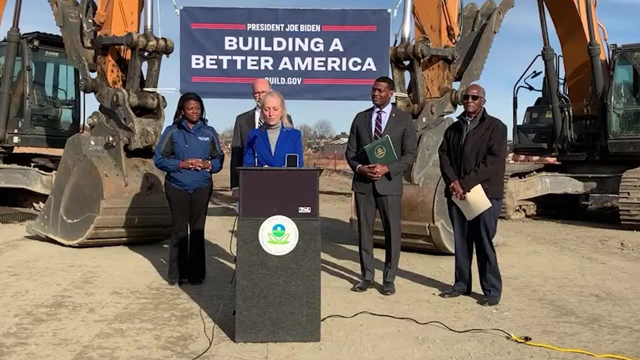 Good afternoon everyone and welcome to Pennsylvania's fifth congressional district. I am so honored to be here today with EPA Administrator Michael Regan, Governor Tom Wolfe, Representative Regina Young and members of the Eastwick- Lower Darby Creek Area Community Advisory Group to celebrate how the recently passed Infrastructure Investment and Jobs Act will help.